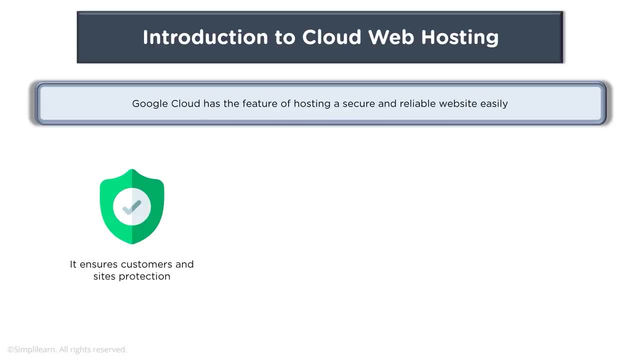 reliable websites easily. It ensures customers and sites protection. The website is a is hosted on a fast and reliable network. You can do more work for less price with Google Cloud. Now, when we talk about Google Cloud, it is always good to know some basics of cloud computing. 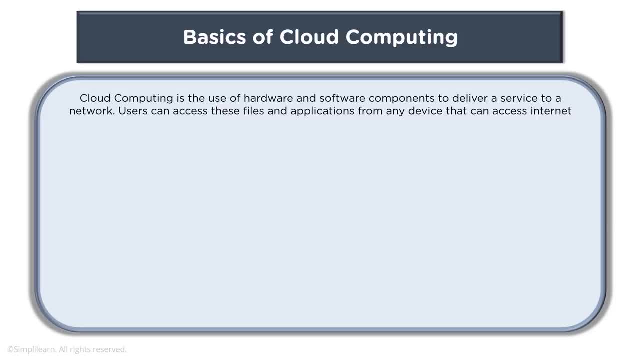 Now, when we talk about cloud computing, cloud computing is basically using resources which are provided by your cloud service provider, such as Google Cloud, and cloud computing basically means cooked cloud that can execute anrell services, usb capabilities, and this centers on your本当 users can access files, applications, from any devices that can access internet. When we talk about 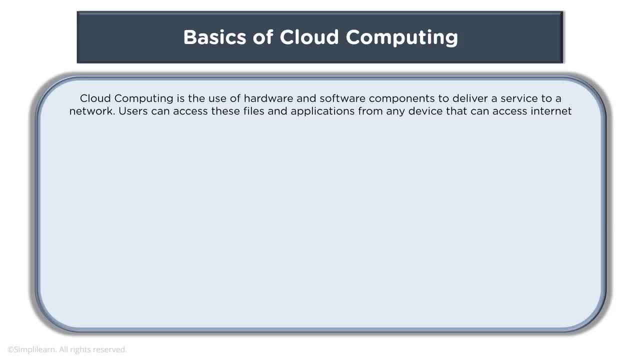 cloud computing, this is basically using services that are revenue hosted on an infrastructure which is managed by a cloud provider. when we talk about resources that can be used, that include big data services, storage, firewalls, network, our cloud web hosting system includes a lot of. 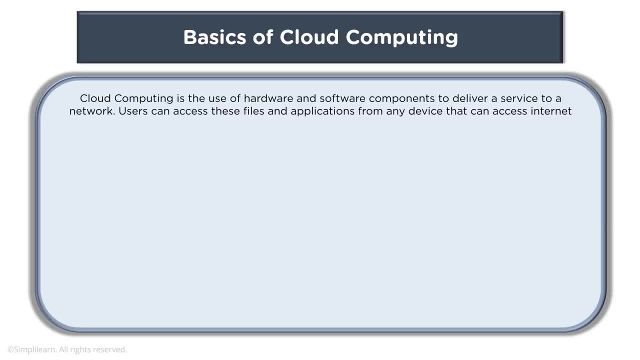 different, different things like openspaces, applications, cloud devices and even �thing storage options, your computing options, networking options and various other services which a cloud provider offers. cloud computing has various different service models, such as you have platform as a service, software as a service, infrastructure as a service also these days. 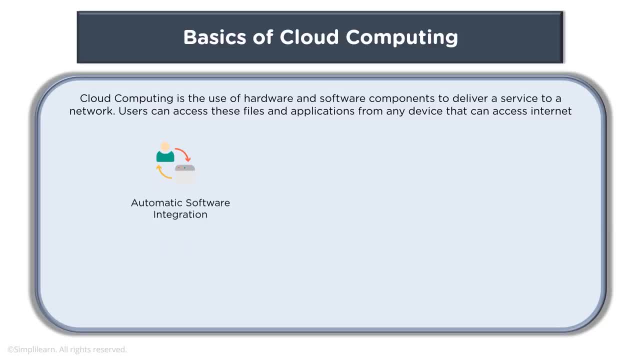 we talk about containers as a service, and these are your different computing service models, which are being offered by cloud service providers, which allow you for automatic integration with your existing environment or, if you would want to benefit from modernization by using a cloud providers infrastructure. you have different services which are offered. some of them are for: 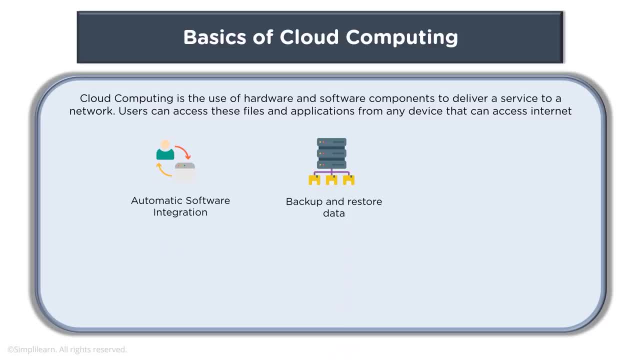 auto software integration or migration. backing up and restoring data. scaling your storage capacity- that is, going for an unlimited storage capacity- and using a resource provided by cloud service provider, benefiting from reliability, cost efficiency, which is offered by a cloud provider. in this case, we are talking about google cloud. when you talk about web hosting service providers. 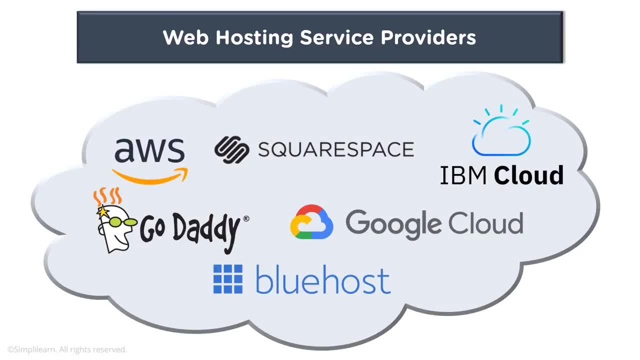 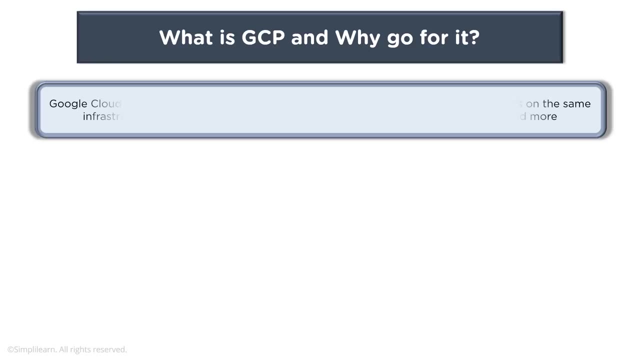 there are various web hosting service providers. you have aws, you have squarespace, ibm cloud, godaddy, bluehost and google cloud. so what is gcp and why go for it? when you talk about gcp, or as we call it, as google cloud platform, it is set of cloud computing services provided by google that runs on the same. 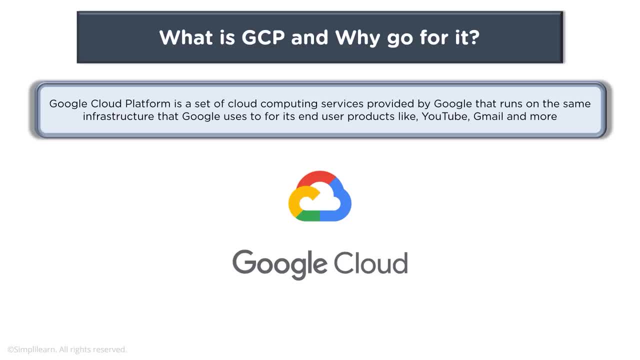 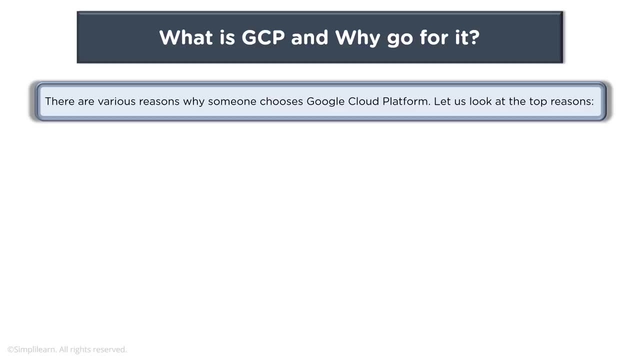 infrastructure that google uses for it, end user products like youtube, gmail and much more. when you talk about gcp, there are various reasons why anyone would choose it for their use cases. now let's look at some reasons. when you talk about pricing, gcp has better pricing compared to its. 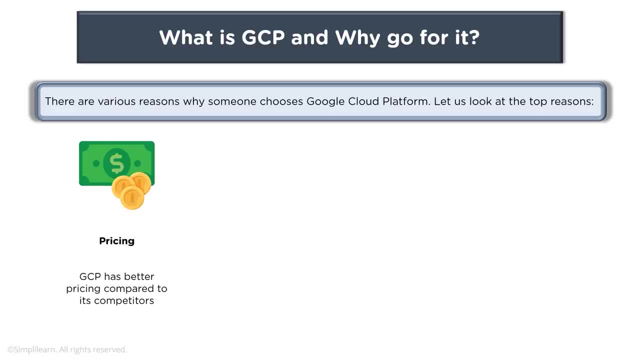 competitors, depending on the services which you would use, whether that would be infrastructure as a service, such as using compute engine instances and running your applications on them, or might be a managed service, such as dataproc or bigtable or your bigquery, where you can have your hadoop clusters. 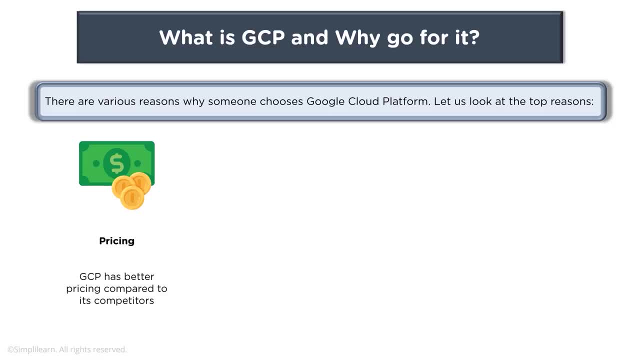 running or store huge amount of data, or even build your data warehouse wherein you can store structured data. so there are different services which gcp offers, and pricing has been a better option in case of google in comparison to other competitors. when you talk about speed and performance, it's very fast and increases the performance of your project if you use different. 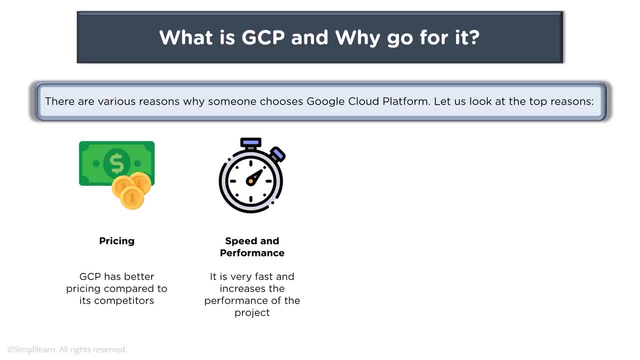 services offered by google. when you talk about migration of apps, this is one of the features which organizations usually like, which none of other competitors are offering when it comes to live migration of apps. so there are specific features. for example, when you talk about compute engine, there is a feature stating live migration. 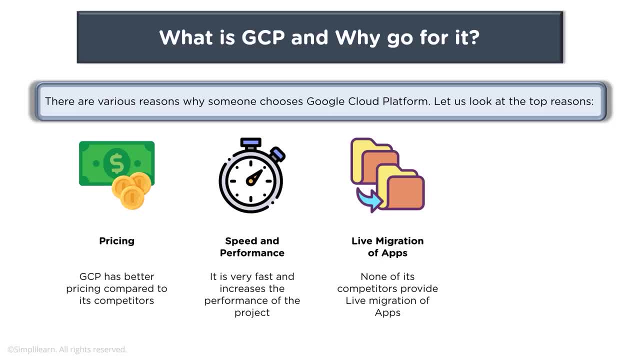 wherein your resources or your instances which are running applications would be migrated during, say, maintenance, from one underlying host to another underlying host without affecting your application's performance, and you can benefit from that. when you talk about big data, google cloud has various offerings in big data space. 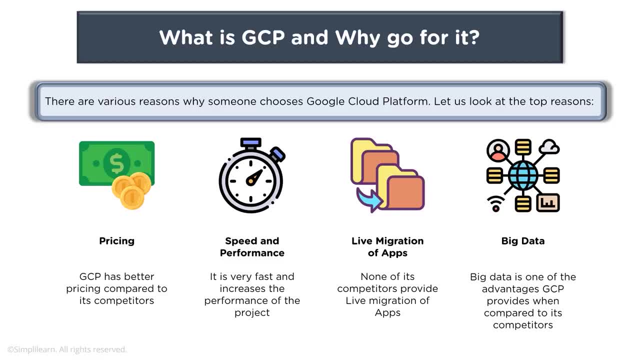 and that's one of the advantages of gcp in comparison to other competitors. you have different services for your big data needs, such as pub sub for publish subscribing messaging system, or going for data proc, which basically allows you to spin up your hadoop and mark clusters to run your different jobs and so on. so when we talk about features of google cloud, 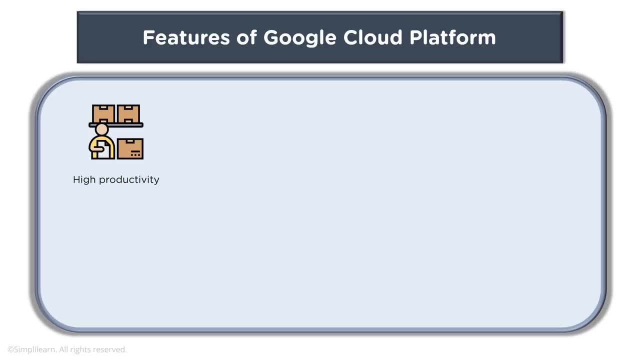 platform. it offers high productivity because you are using the resources which are based on the same infrastructure which google uses for its own different use cases. you can work from anywhere, provided you have internet connection and you can connect to the cloud platform and use different services offered via web. you can quickly collaborate with the cloud. you can connect to cloud services. 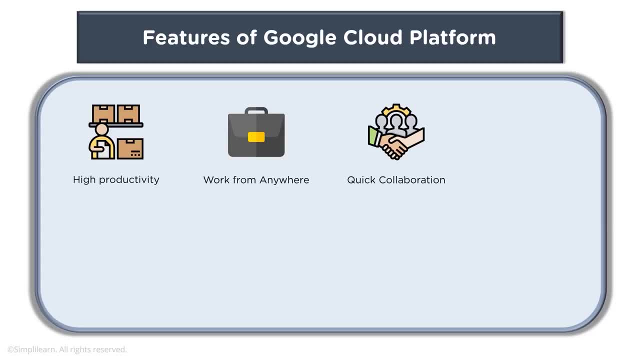 different teams or different colleagues working on different projects which might be sharing or using different GCP resources. You are benefiting from high security and different encryption and security mechanisms which GCP offers. Now there are fewer sources, or you could say data, which is stored on vulnerable devices. There is high reliability, flexibility or scalability, which 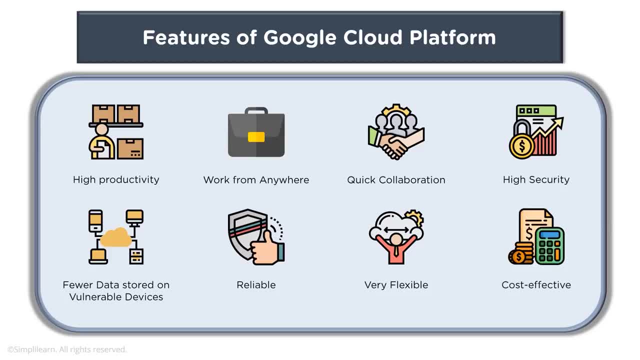 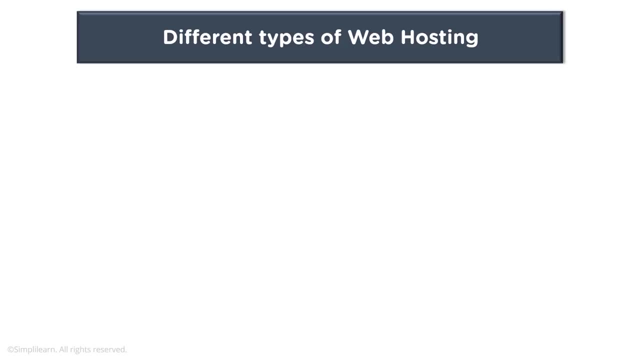 GCP offers and the cost effectiveness really makes it as a good choice when you would want to benefit from infrastructure modernization and using a cloud platform solution for your use case. Now, when you talk about different types of web hosting, Google Cloud offers three types of web. 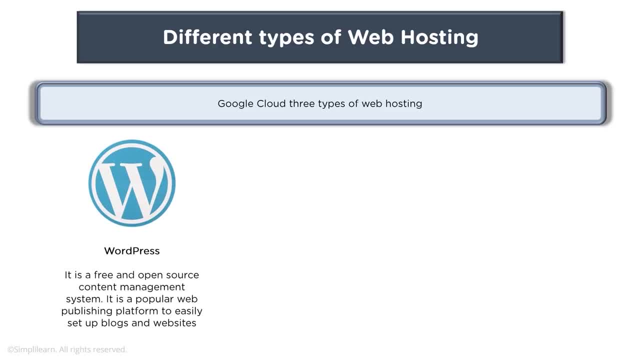 hosting. You have WordPress Now. it is a free and open source content management system. You might have used in past or have heard about WordPress. You might have used GCP Now you might have used WordPress, where a lot of websites are being created. It is a popular web publishing platform. 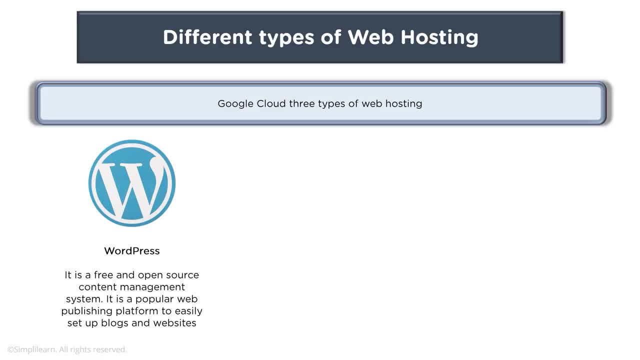 to easily set up blogs and websites and thus used by organizations or even individual users for having their blogs or running their websites or promoting their products. You have LAMP, which stands for Linux Apache, MySQL and PHP, and LAMP stack consists of Linux Apache HTTP server. 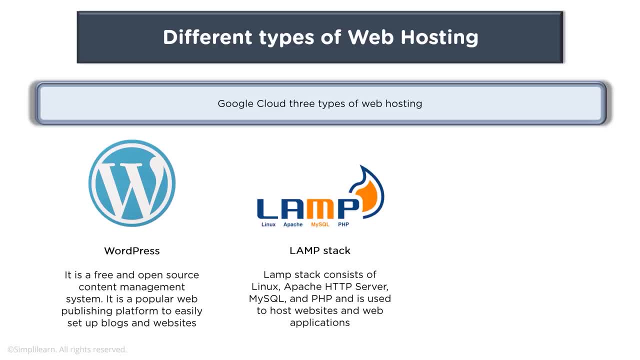 MySQL and PHP and is used to host websites and web applications. You also have your option of building your own website, so you can develop website or web application with your own code directly on Compute Engine. Now let's look at a use case and understand what happened here. when we talk about 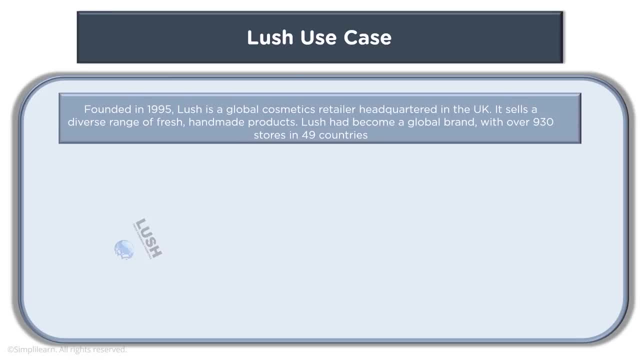 Lush. So Lush was founded in 1995.. You might have seen this brand somewhere in the streets. It is a global cosmetics retailer headquartered in UK. It sells a diverse range of fresh handmade products. Lush had become a global. 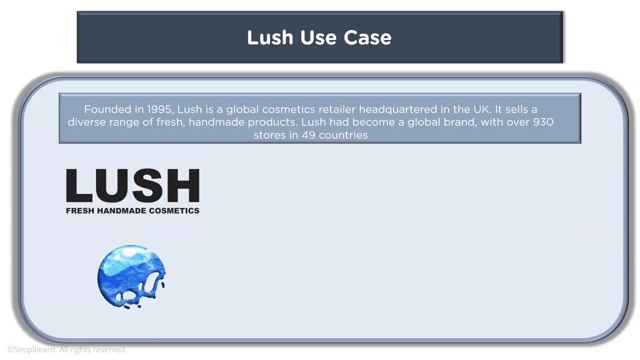 brand with over 930 stores in 49 countries, So the challenges which were faced here was traffic on Boxing Day caused website crash for almost 18 hours, and this is something which had a devastating effect on their business. The previous platform had no scalability option. 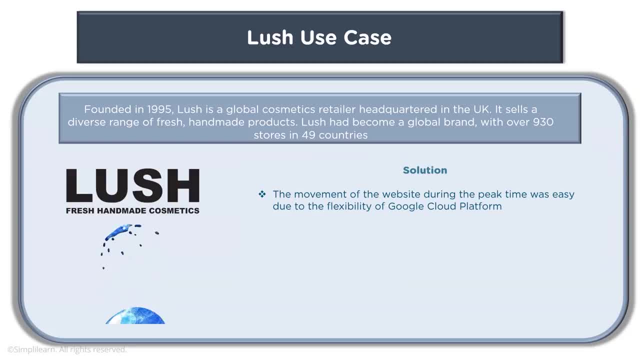 What was the solution? The movement of website during the peak time was easy due to flexibility of GCP platform, With rapid VM deployment on Google Compute Engine. the environments were monitored and destroyed in minutes so the team could test and deploy at speed By using Google Cloud SQL. Lush took complete control of its infrastructure and 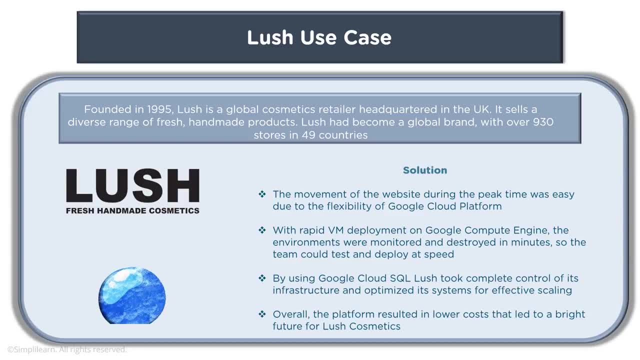 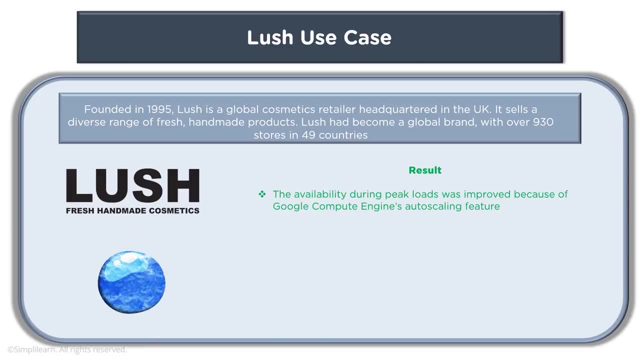 optimized its systems for effective scaling. Overall, the platform resulted in lower cost. that led to a bright future for Lush Cosmetics. Now, what was the result of all this? The availability during peak loads was improved because of Google Compute Engine's auto-scaling. 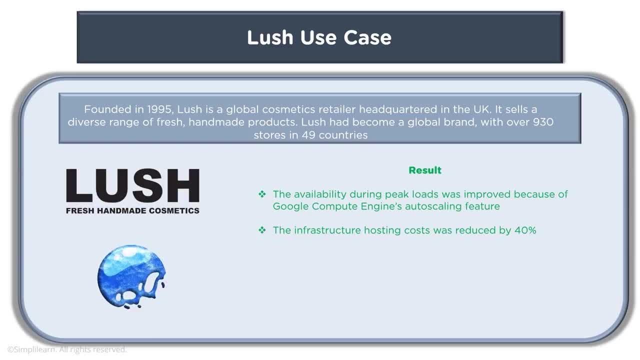 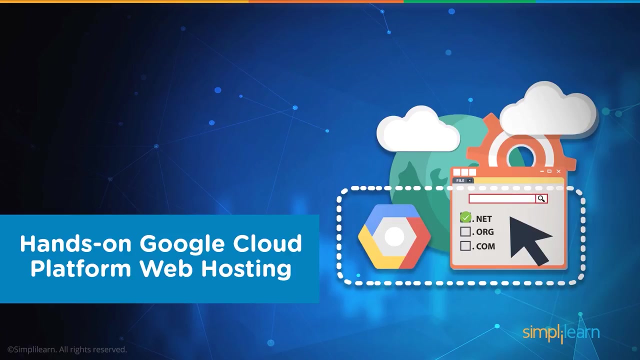 feature. The infrastructure hosting costs were reduced by 40%. Streamline data center usage from 5 to 3 with Google's high-quality private network really benefited Lush, and it provided a flexible architecture and scalability for future business growth. Now what we have seen here is that your Google Cloud and its web hosting basically offers users. 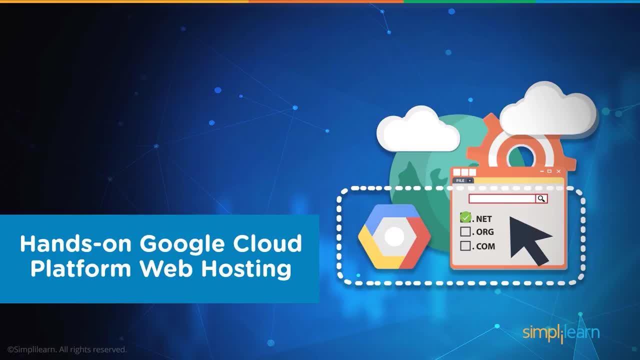 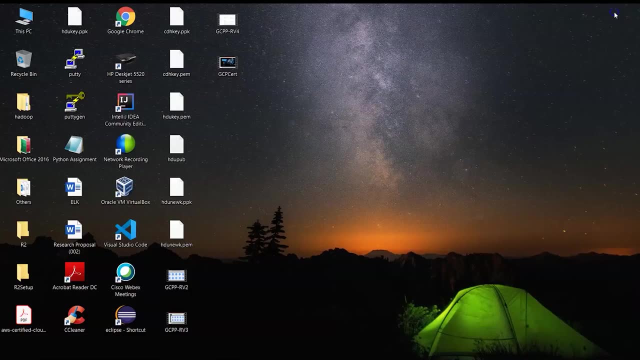 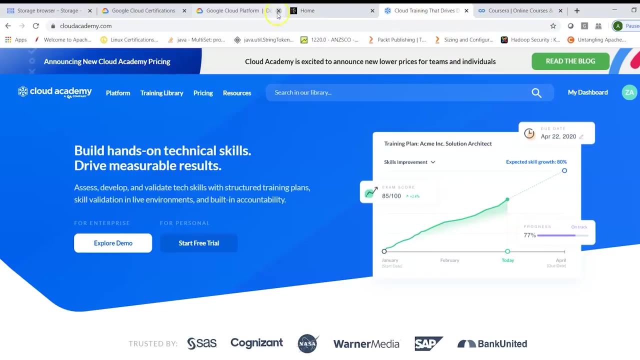 to run their websites or use a web hosting solution that can benefit in more than one way. The simplest approach could be seen is by clicking and setting up a VM instance by going to your console. For example, if we go in to the Google Cloud platform clicking on console. 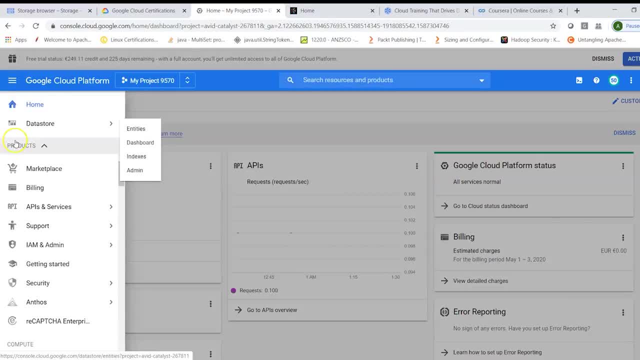 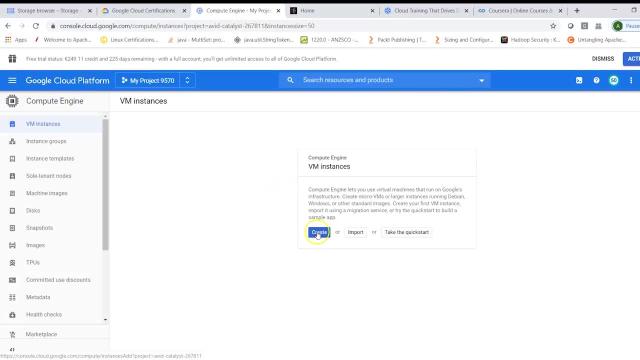 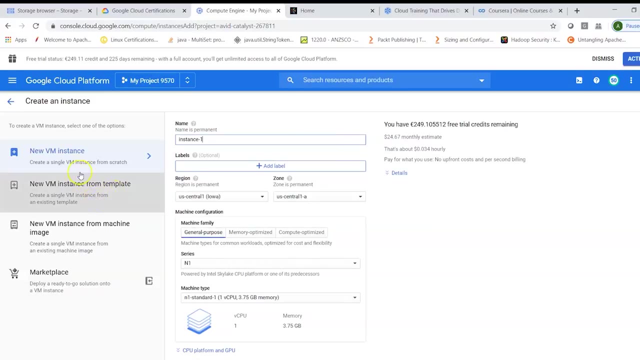 here. the easiest way I could test it is by going to my Compute Engine VM instances and here I can spin up an instance I can click on create Now. in my previous sessions I have also explained about how you could create a template and run an instance from that. 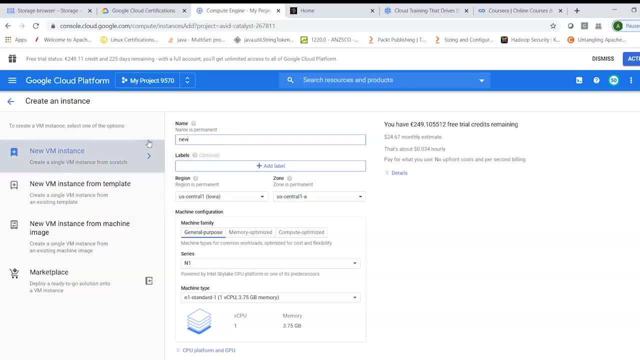 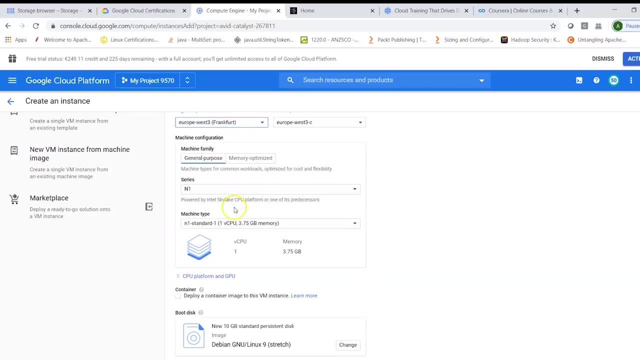 We can also click on new VM instance. Let's call it new instance. I will choose a region, For example Frankfurt. I will let it be general purpose. For example, I will let this machine be one virtual CPU core and 3.75GB RAM, If I am looking. 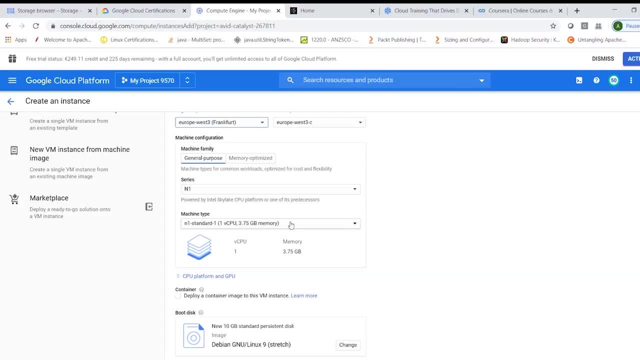 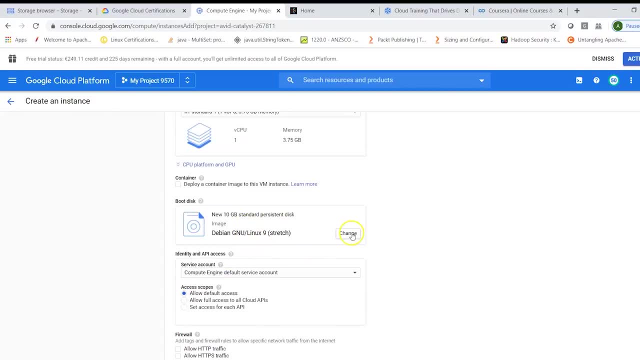 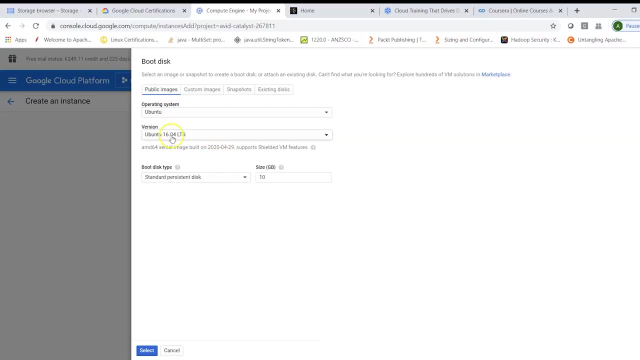 for a heavier website which might have more users logging in and so on. then I can choose a higher configuration machine. Here we have the option to choose our distribution. So, for example, I can choose Ubuntu and then I can choose a distribution version. So let 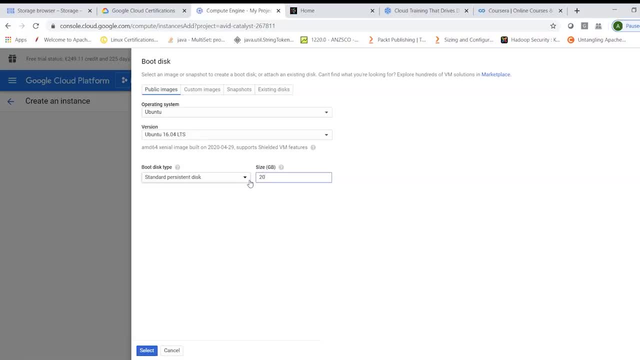 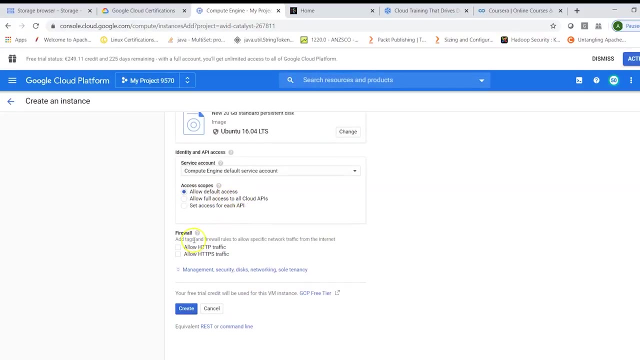 it be 16.04.. We can choose the disk size to be 20GB And we can use SSDs or HDDs. So as of now it is standard persistent disk, That is HDD, and that should be enough. Let's click on select. Here I will say allow default access. 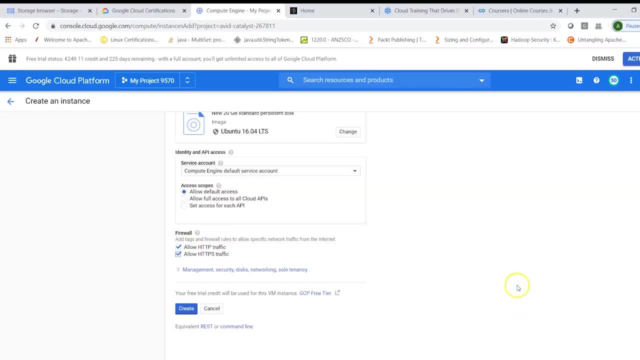 I would say: allow HTTP and HTTPS, so that if I have a website content hosted on this machine, I can access it over HTTP. Now, here you have management options for your instance. You have security option, which basically allows you to access your instance. So if I want 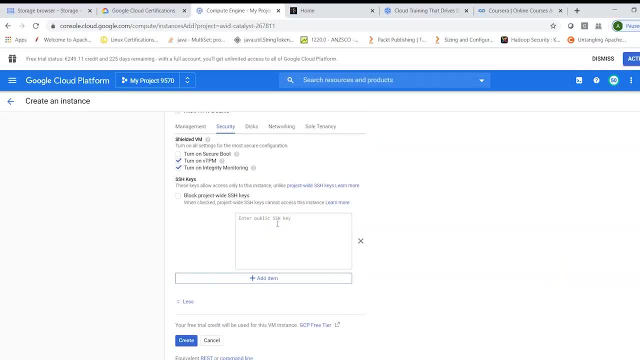 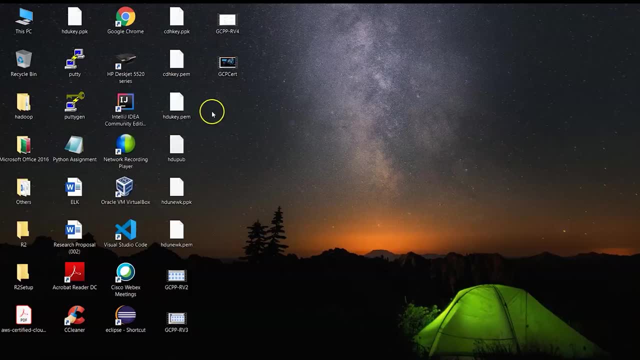 to access to a public key. I can choose to access the public key or if I want to access a private key, I can choose to access the private key. In the same way, I have created a private key which is here. I have also converted. 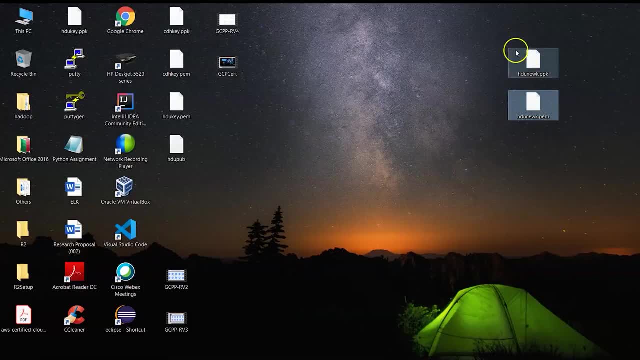 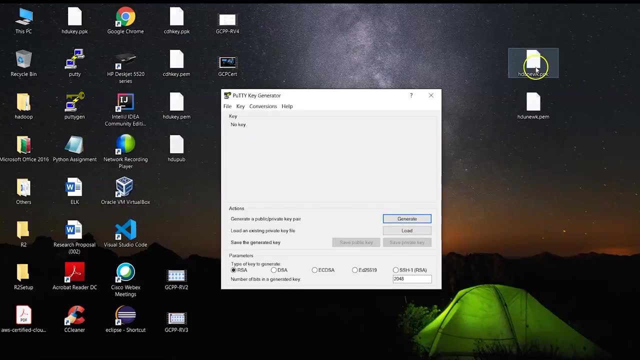 that as a PEM file and anytime if I would want to use this key, all I need to do is click on puttygen, where I had earlier created this PPK file. Now I can just do a load and I can choose the key which I have here. 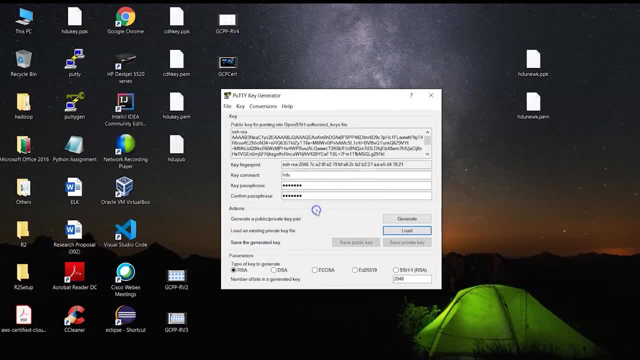 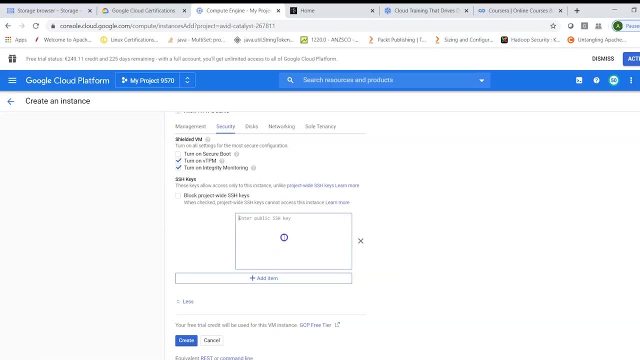 and I can give the pass face. click on ok and that shows you the public key. let's copy the public key from here. let's go into our instance and I can give this here. that resolves the name. so I have the private key saved on my machine and 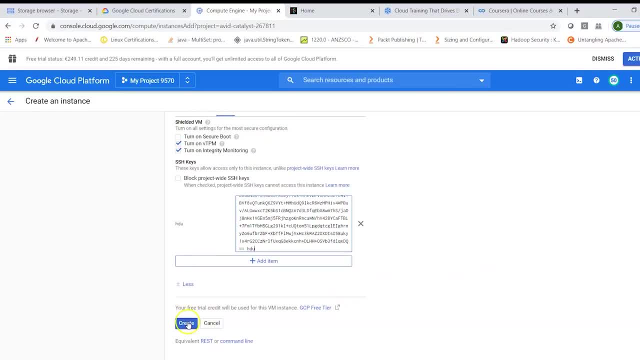 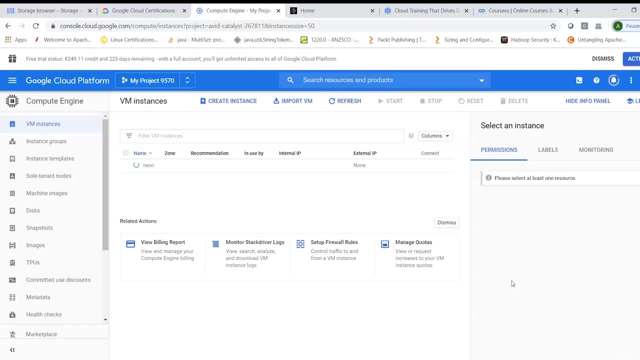 public key which will be pushed into the machine. I can click on create, and that should create my instance, to which you can connect using SSH from the console itself or using a external client such as putty, which will then need the public IP of this instance, the PPK file, what we have and you can connect to this. 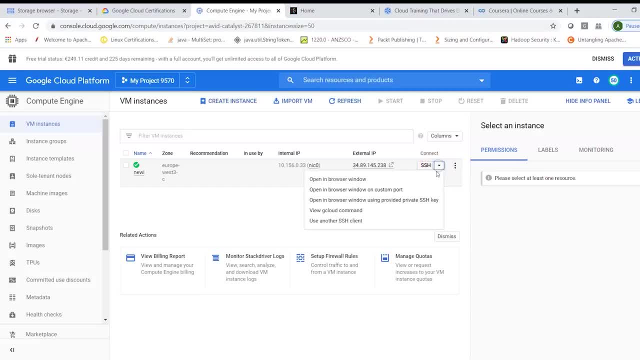 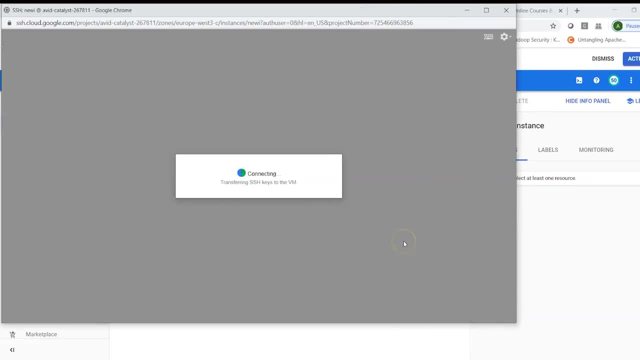 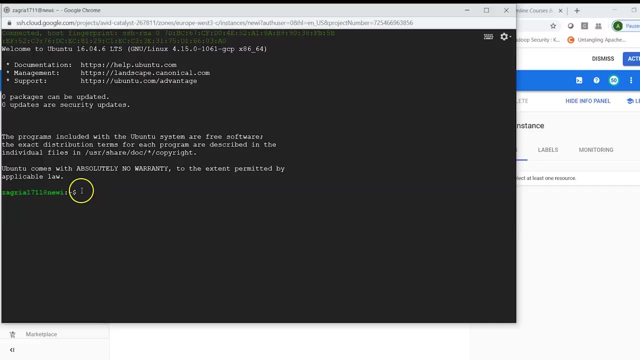 instance. what I can also do is I can just do a simple SSH from here, and that will basically allow me to connect to the instance. what we also need to remember is each instance, what we create in compute is also having some default firewall rules. now I have connected to my instance. 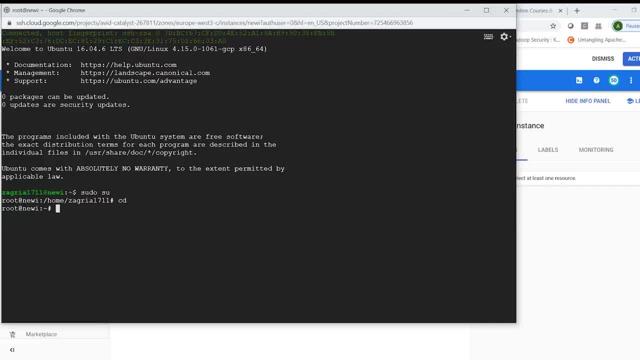 you can see that I have connected to my instance. and now I have connected to my instance, I can click on sudo, su, I can log in as root and here, if I would want, I can install a particular service. so let's say Apache, let's say apt-get. 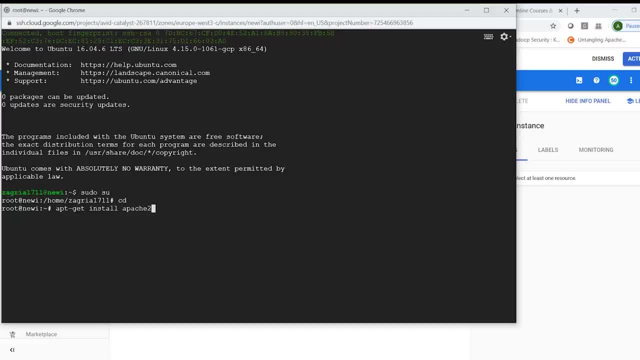 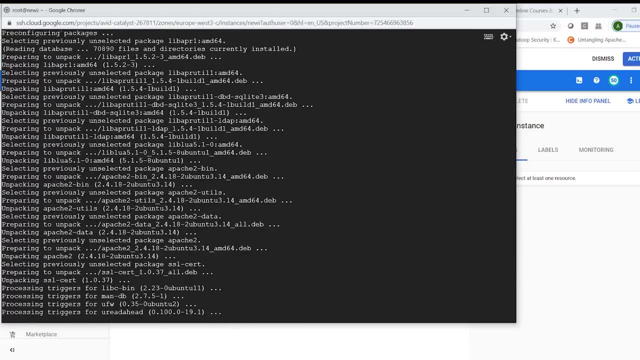 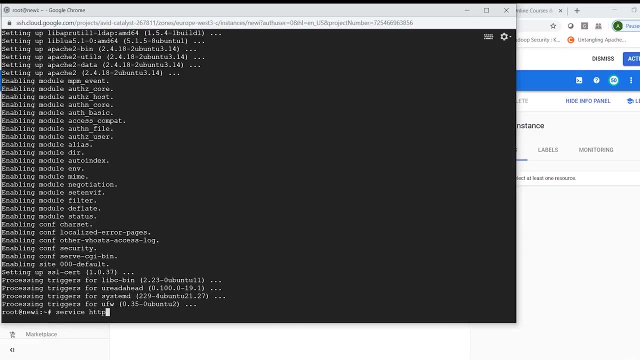 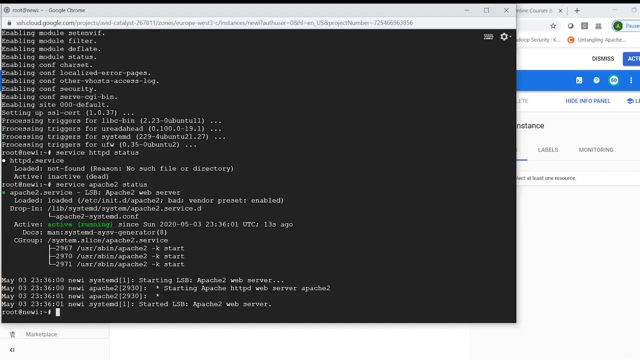 install and then I can say Apache 2 or HTTP D, that is basically to host your web application. so I'm installing the service and here I can check if the service is running by doing a service HTTP D status. or I can say service Apache to status, which says it is already running. 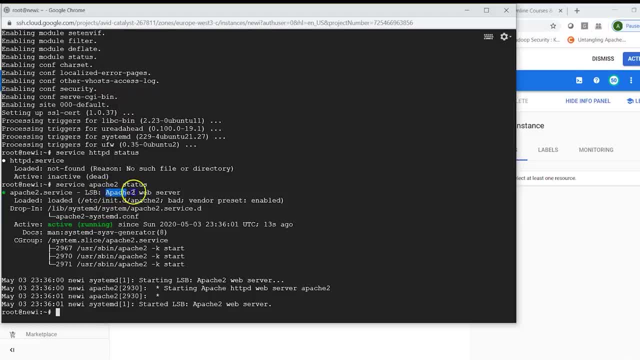 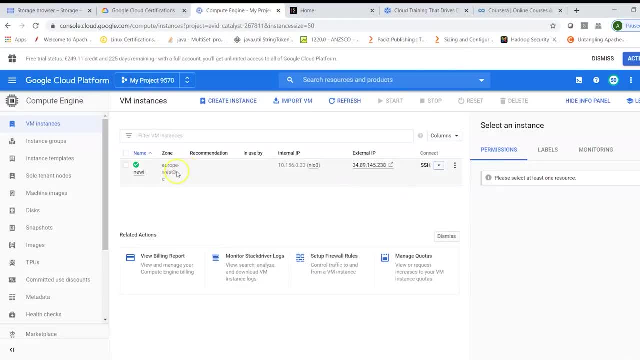 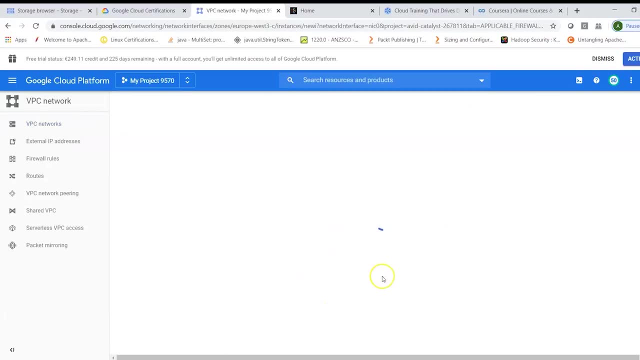 that means the Apache web server page will be accessible from HTTP, provided my firewall rules allow that. now, before we look into this, we can also, for our instance, look at the firewall rules. so here you have network details. now, since we created an instance by default, Google has created some firewall rules, which. 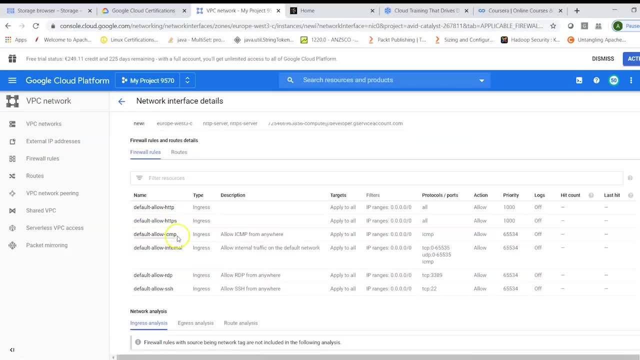 allow default HTTP D and header-to-header password, HTTPS, ICMP, your default internal access, RDP and SSH access. and here it says these ingress rules which allow incoming traffic are allowed from anywhere. We can customize that at specific IP addresses. We can also look at egress, which is basically outgoing traffic, and this is again. 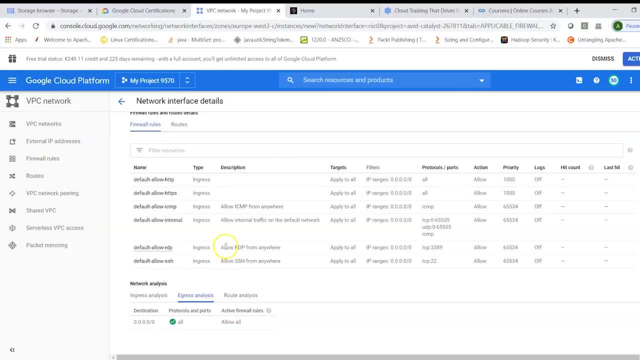 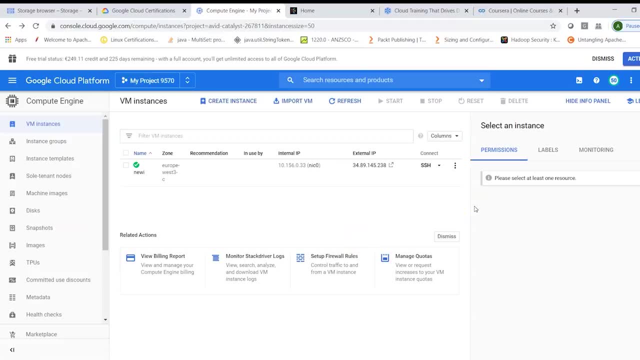 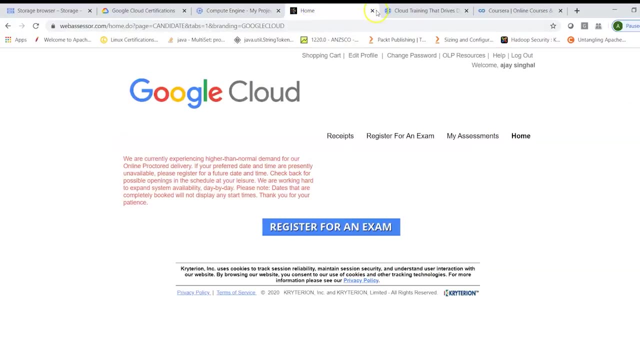 saying: my machine can connect to the external world in different ways, using different protocols, So you can customize these firewall rules As of now. I'm going to let it be default. Now we connected to our instance from the browser and we were basically checking how you can use this. 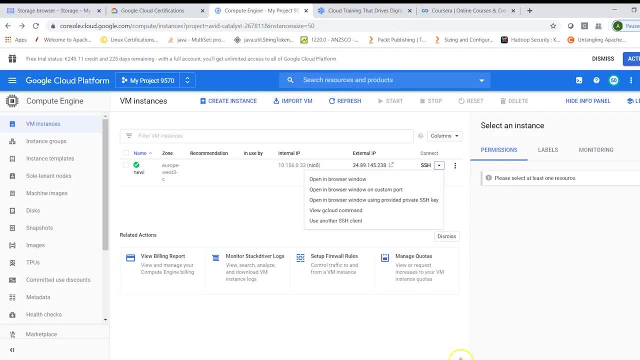 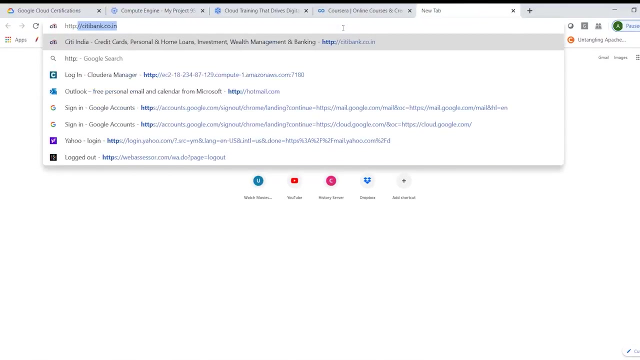 browser by clicking on this. Now, what I can also do is here I'm logged into the instance My Apache server is running. So the best way to check if the Apache web server is accessible via HTTP all I need is my public IP. So let's copy this, Let's go here and I will say HTTP: slash, slash, Just give your. 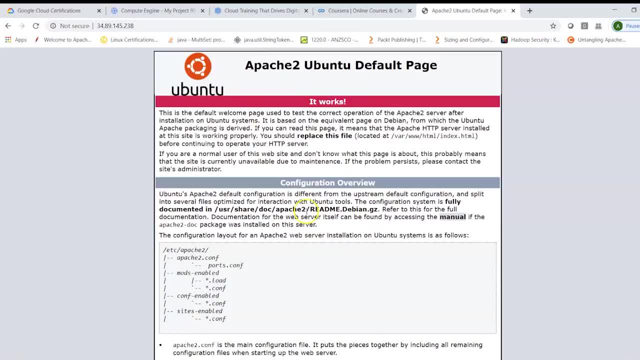 public IP and that shows your Apache 2 web server page. That means the Apache service has already been run. Now here it tells if you would want to host a particular page. what you will have to do is as it says here. it is based on equivalent page on. 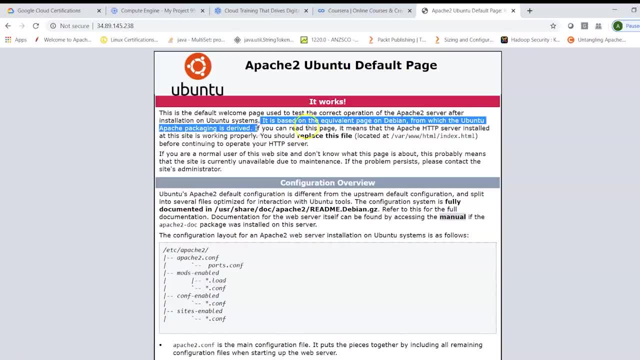 Debian, from which Ubuntu Apache packaging is derived. If you can read this page, it means Apache HTTP server is installed at. this site is working properly. Now you can replace this file located at var- wwwhtml- indexhtml before continuing to operate your HTTP server. So. 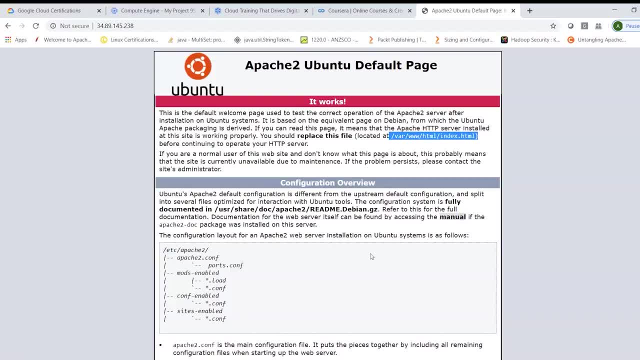 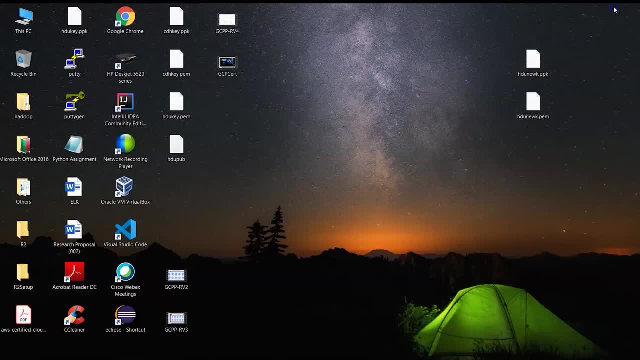 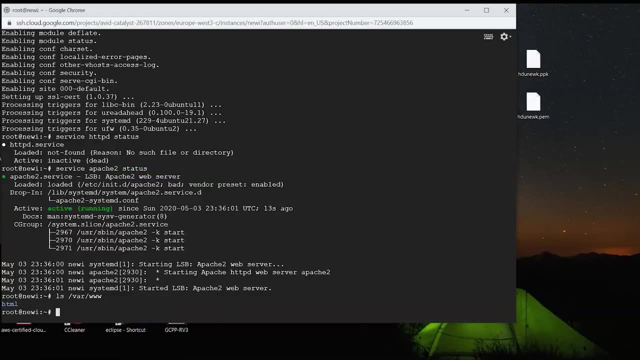 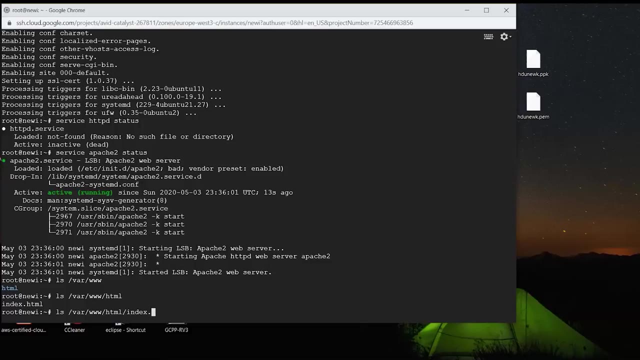 this is where you can change the particular page and you will be able to host your web site on this particular. What we can do is we can check this, So we can go into the browser and we can look in var www and that has an HTML folder. Look into this and, as of now, you have a indexhtml and that, basically, is. 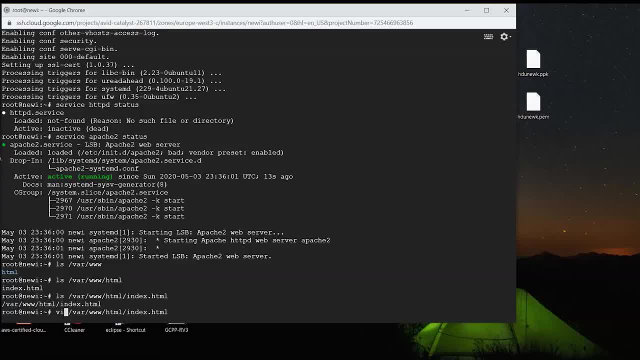 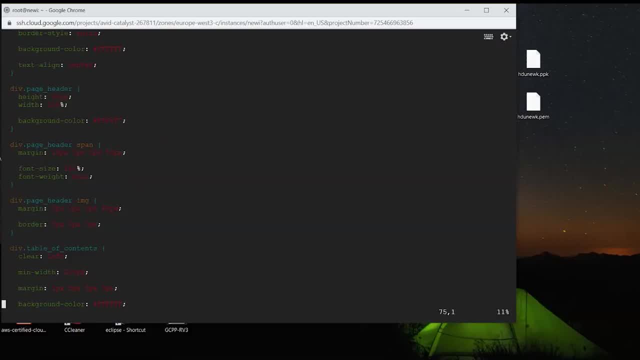 the page what we are seeing. Now I can click on this one and I can see I have a small HTML page which is basically showing me what we are seeing On our web server. what I can also do is, for now I can test it out and I can put in a different. 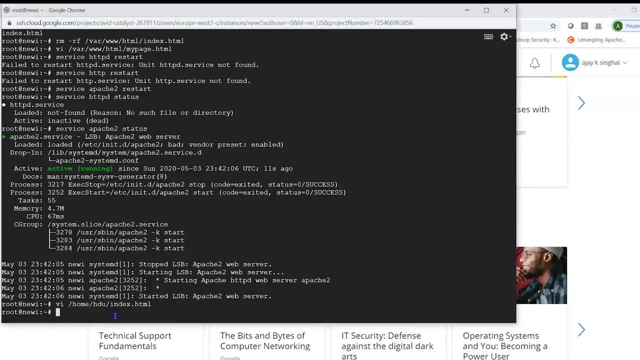 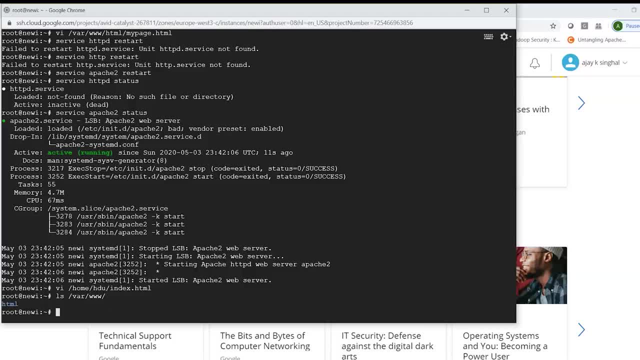 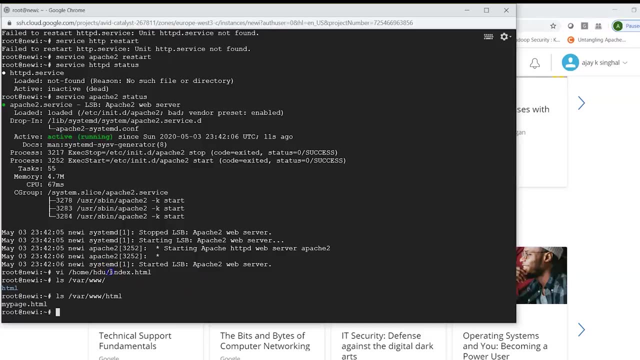 HTML page and see how that works. So we had basically the page here in var www and then we had the HTML folder and in HTML folder what I had was this index file. So as of now, I just moved it and I put it in a different location. So if I look in my browser I can see that I have a 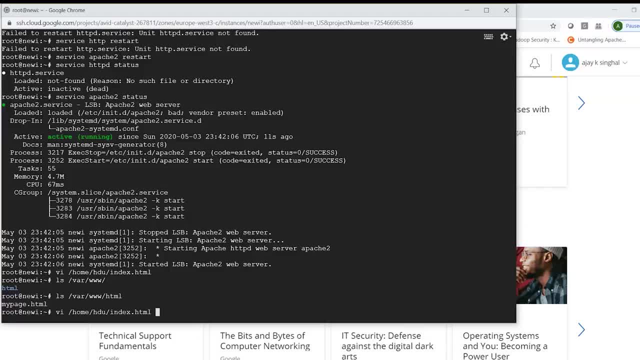 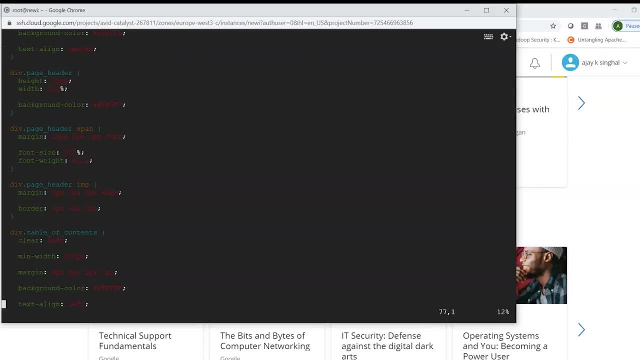 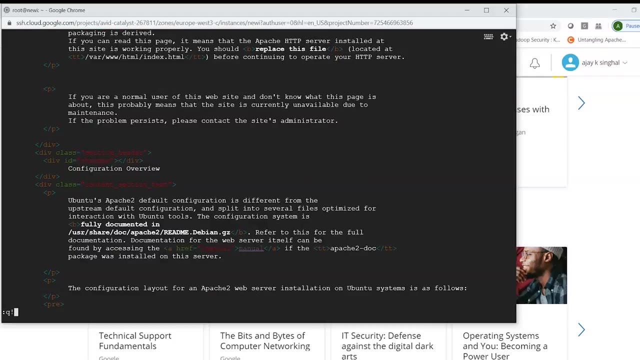 home HDU indexhtml. that shows me the complete HTML page, what we were seeing on our web server. and here it shows you what this page would display if you run it on your HTTP. It says Apache 2- Ubuntu default page. It shows it works, It shows the content and so on. So for just 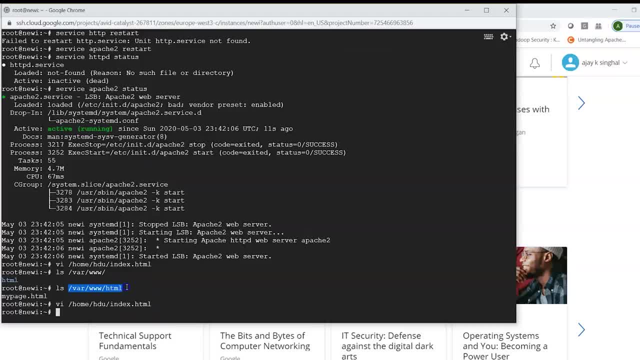 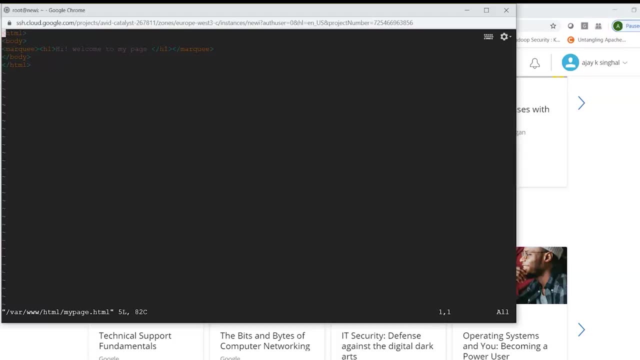 testing. I moved this page out from this location and what I did was I moved this page out from this location and I added a different page here. So that page, if you look in HTML and then look in my pagehtml section, I've just added some basic details of creating HTML. I'm saying body, I'm 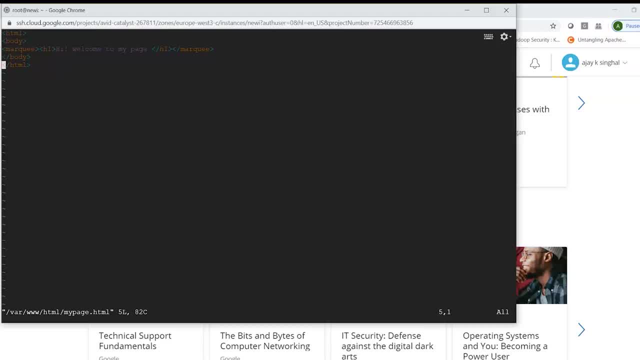 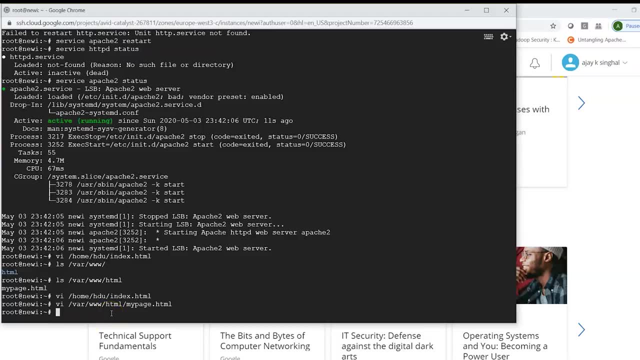 using marquee and then I'm closing this with HTML tag. Now, this is a simple HTML page which I created, and now what I did was, once I've done this, I basically did a service Apache start. So once you do that, it will take up your new page. and once you have done that, now you can. 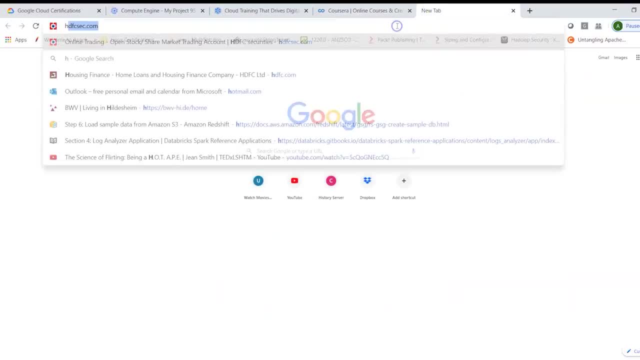 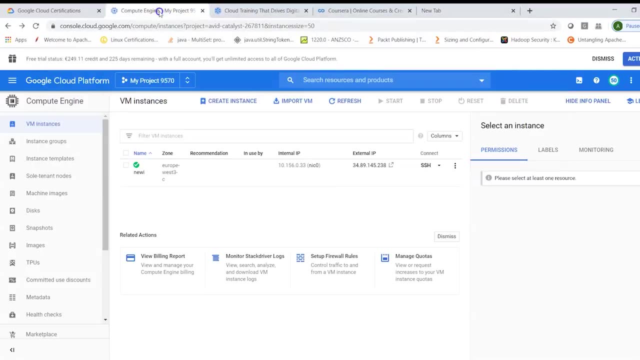 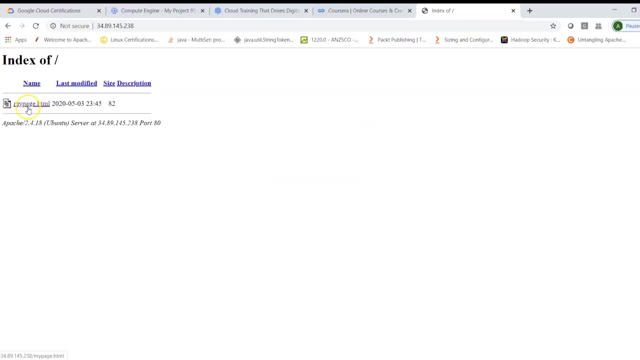 access that by going to your HTTP, give in your details and then basically give your public IP, which we can get from here, and just paste it here Now. hit on this So that shows me there is a mypagehtml. I can click on this and that basically shows the simple page, which is: 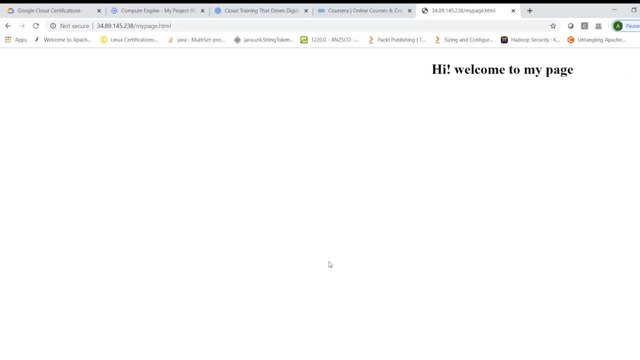 I created. So, as of now, this is my web page, which I've created, and this is hosted on my compute instance. Now, obviously, we can create a more complex website backed up by a database. use PHP, use MySQL to store the data and then host your website on a Google Cloud Platform service, such 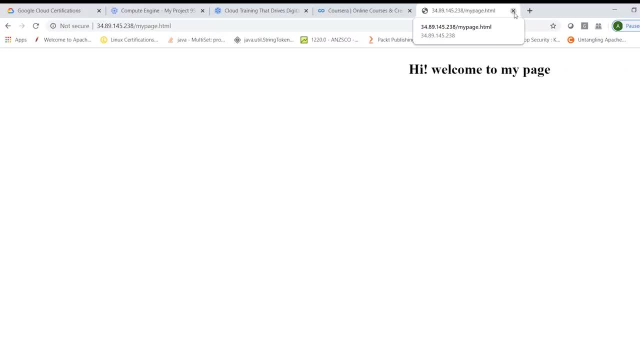 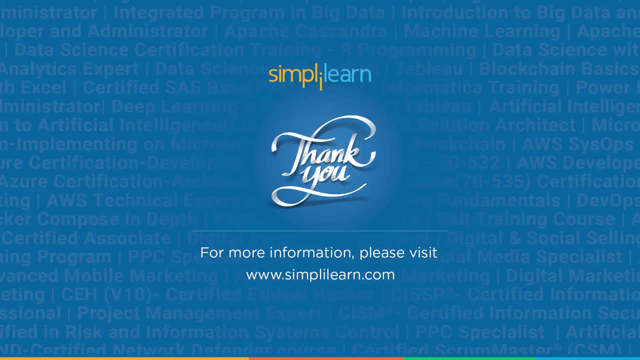 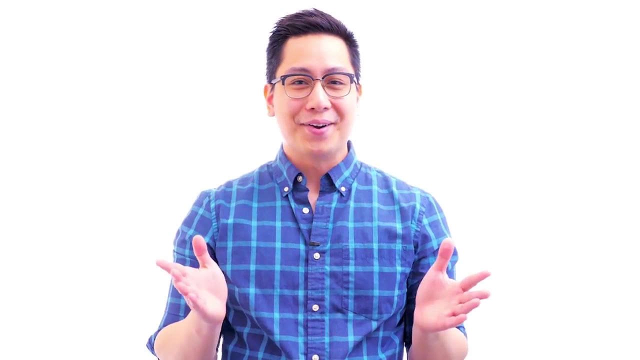 as compute where your actual code is running, So we can learn about your web hosting on compute instances in further sessions. Thank you, Keep learning Hi there. If you like this video, subscribe to the Simply Learn YouTube channel and click here to watch similar. videos To nerd up and get certified: click here.